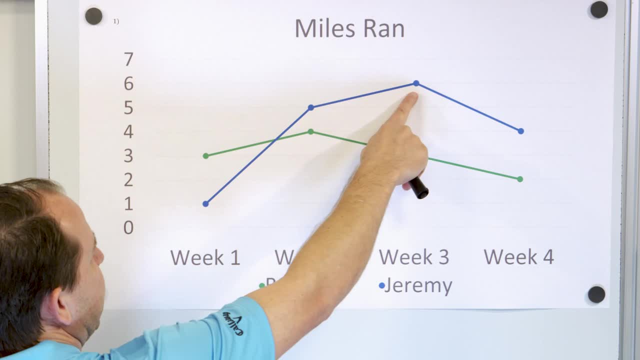 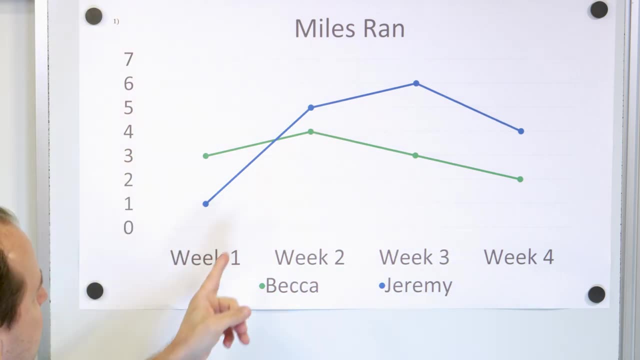 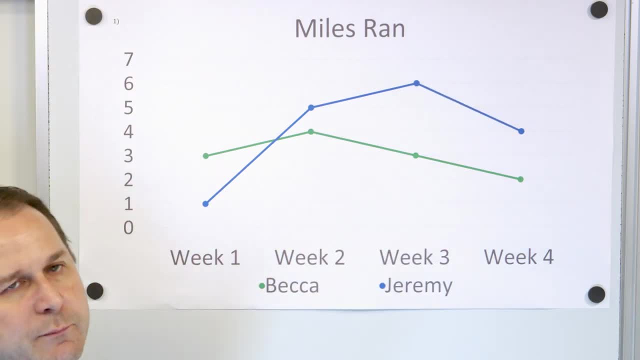 ran more, Jeremy ran more. It's only in the first week that flipped around Becca ran more. So what does that mean? Maybe Becca just didn't have much time, Who knows why. They just didn't, you know. 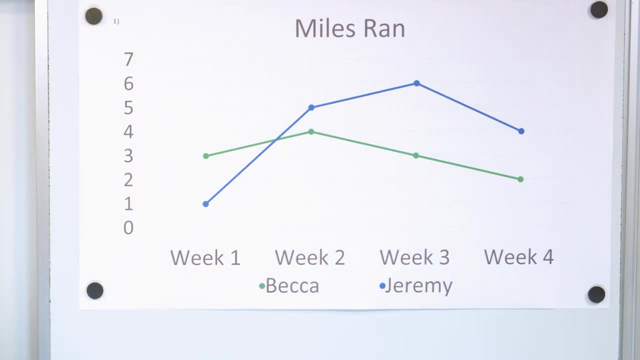 they just have different schedules and he had more time to run, or something like this. But that's how you actually read the graph: Two different colors. Read the chart over to the right to see how to read it. You go up and you read over. up and you read over, like this: All right, let's take a look. 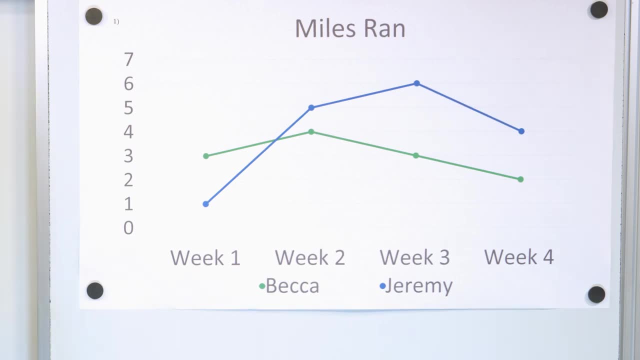 at question number one: On what week did Becca run more than Jeremy? We just answered the question. We have Becca in green right here and Jeremy in blue right here Here. Jeremy ran more. Jeremy ran more. Jeremy ran more. 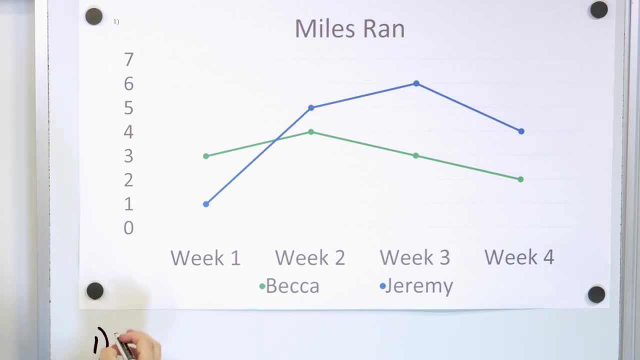 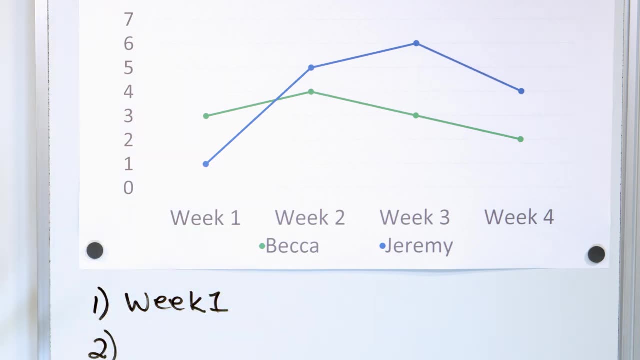 But here Becca actually ran more. So what week did Becca run more than Jeremy? It's week one. Okay, that's the answer to question one. Question number two: how many more miles did Jeremy run than Becca on week three? On week three? So you ignore week one, You ignore week two, You ignore. 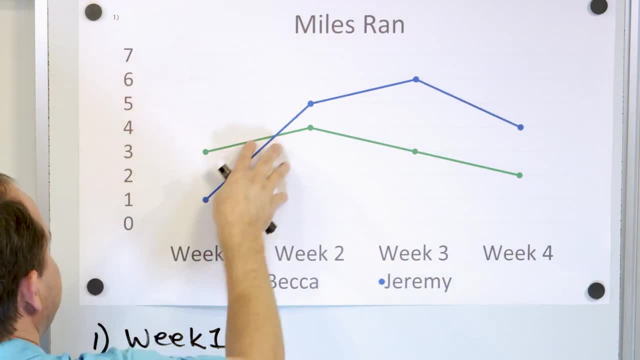 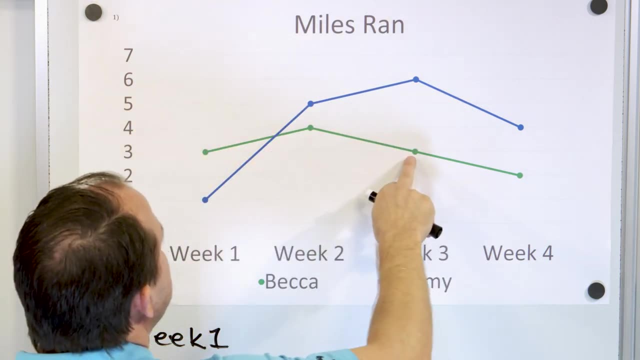 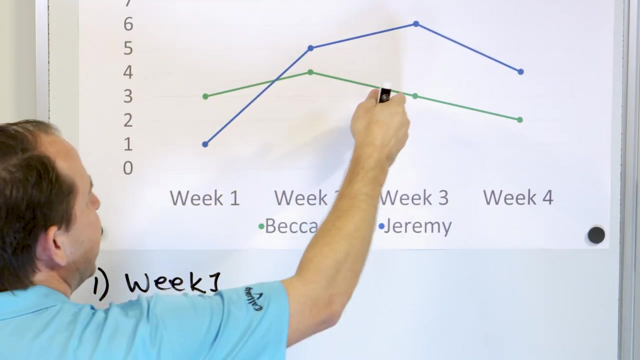 week four And you only focus your attention on week number three. How many more miles did Jeremy run than Becca? Jeremy ran six, Becca ran three. How many more miles? It's just six minus three, right, I could write it down, but six minus three is three. So on this week, Jeremy ran three more. 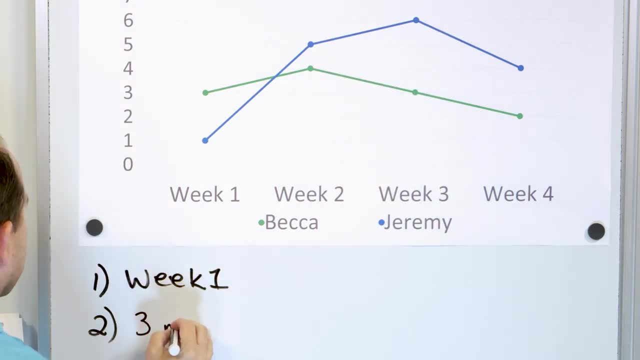 than Becca. So on week three he ran three more miles. Now you might say these are kind of simple problems, And maybe that's true. But the point is, you know you're not going to be able to answer all the questions. You're not going to be able to answer all the questions. So the point of 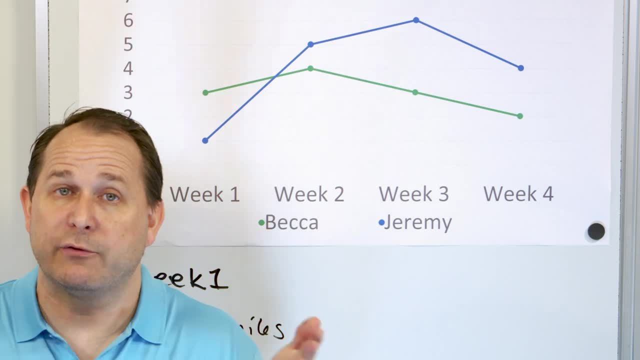 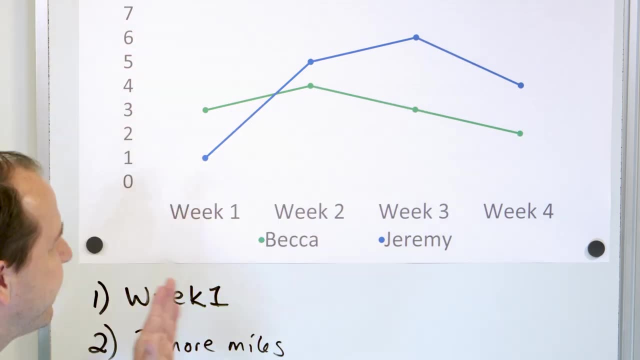 it isn't so much the answers to the questions. The point of it is to know how to read a graph, and especially how to read a graph when you have two or more different lines going on right, And the real secret to it is it looks very busy, but you just isolate it to columns. Week one. this is what. 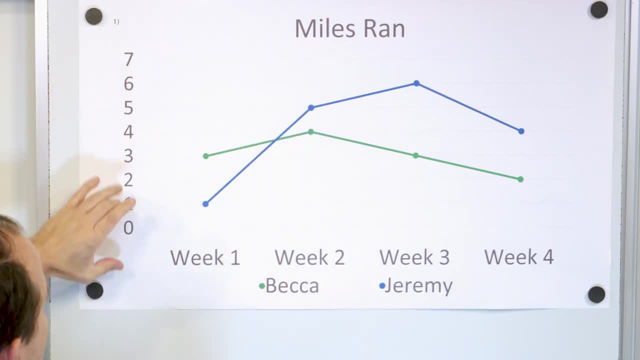 graph: Two different colors. Read the chart over to the right to see how to read it. You go up and you read over. up and you read over like this. All right, let's take a look at question number one. On what week did Becca run more miles than Jeremy, And on what week did Becca run more miles? 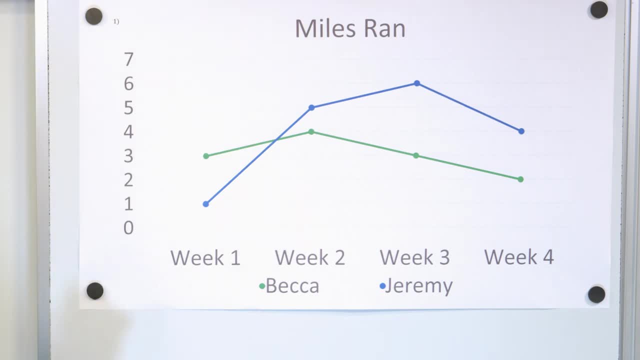 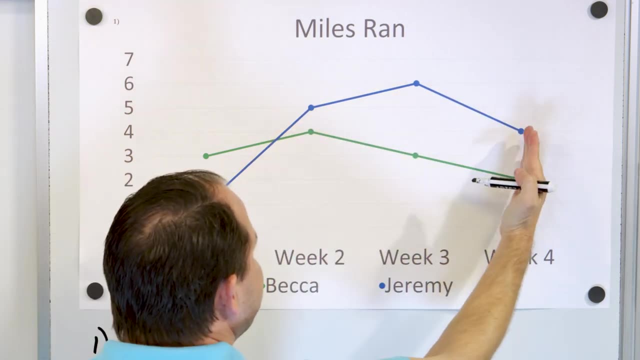 than Jeremy. On what week did Becca run more than Jeremy? We just answered the question. We have Becca in green right here and Jeremy in blue right here. Here Jeremy ran more, Jeremy ran more. Jeremy ran more, but here Becca actually ran more. So what week did Becca run more than? 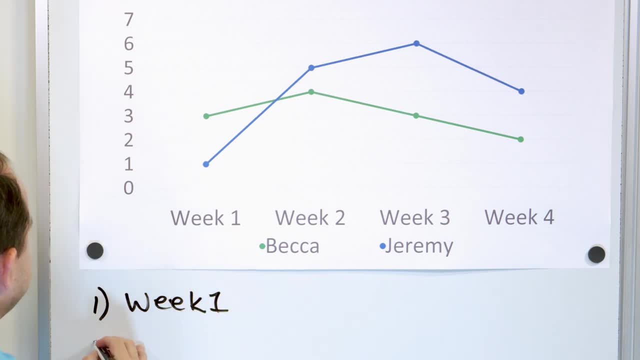 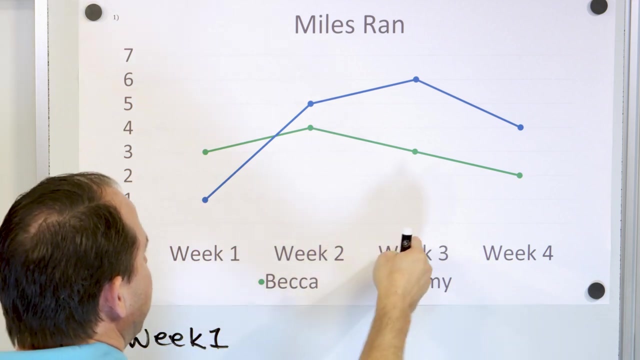 Jeremy, It's week one. Okay, that's the answer to question one. Question number two: how many more miles did Jeremy run than Becca on week three? On week three? So you ignore week one, you ignore week two, you ignore week four and you only focus your attention on week number three. 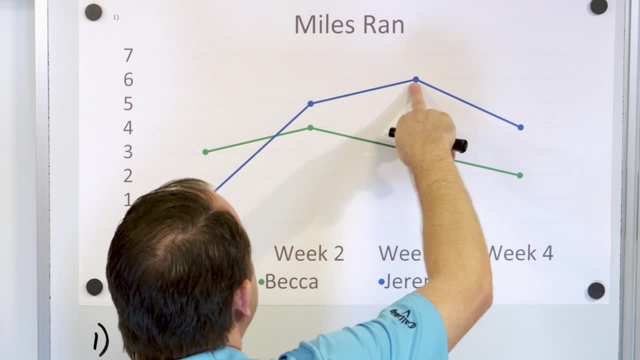 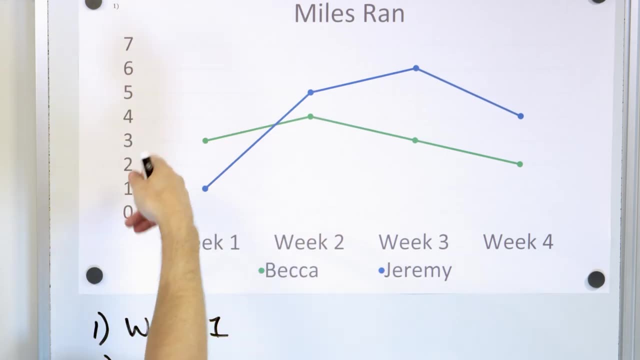 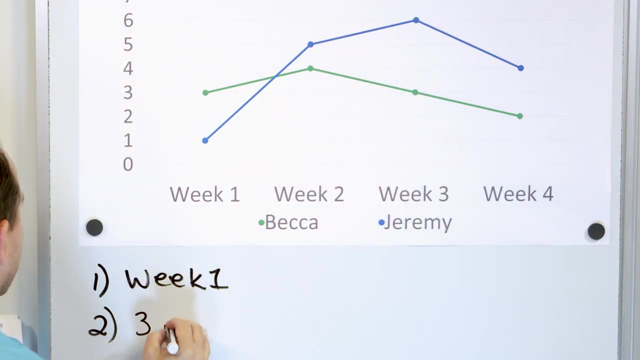 How many more miles did Jeremy run than Becca? Jeremy ran six, Becca ran three. How many more miles? It's just six minus three, right? I could write it down. but six minus three is three. So on this week Jeremy ran three more than Becca. So on week three he ran three more miles. 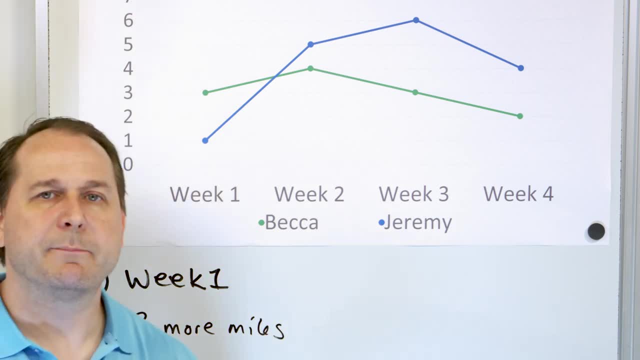 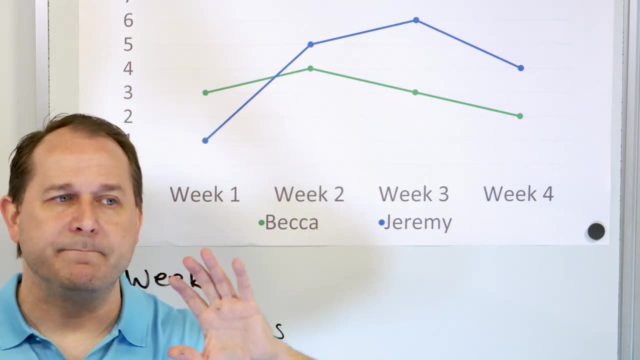 Now you might say these are kind of simple problems, and maybe that's true. but the point of it isn't so much the answers to the questions. The point of it is to know how to read a graph, and especially how to read a graph when you have two or more different lines. 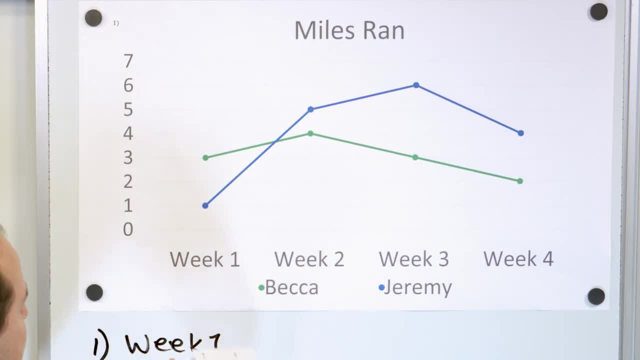 going on right, And the real secret to it is it looks very busy but you just isolate it to columns. Week one: this is what is happening. Week two: you go up, read these numbers, that is what is happening. Week three: you go up: this is what is happening, and so on. And so, if you isolate it, 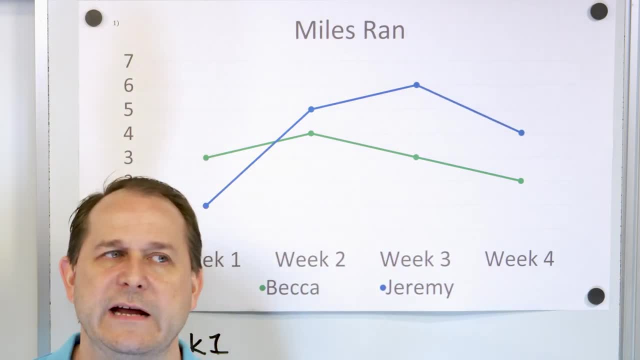 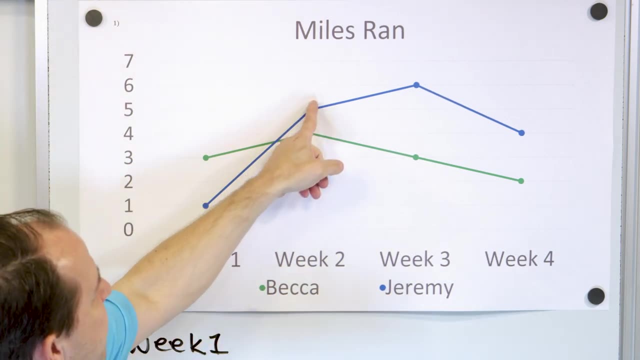 to week one and two and three and just look at what's happening on those weeks. then it makes more sense And you can use the connection of the lines to get an idea of the trend. You can see that in general Jeremy runs more often or more miles than Becca, but of course there's an exception. 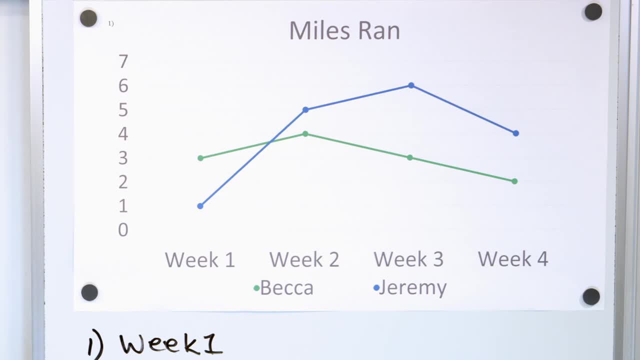 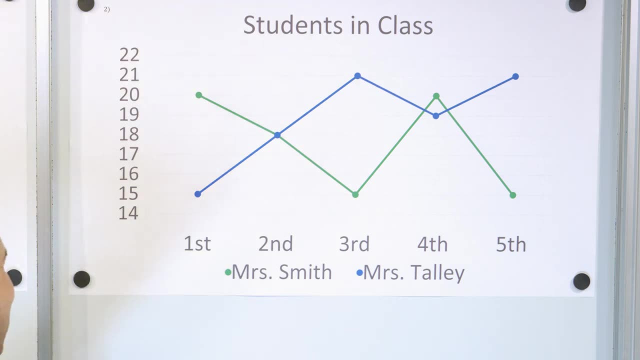 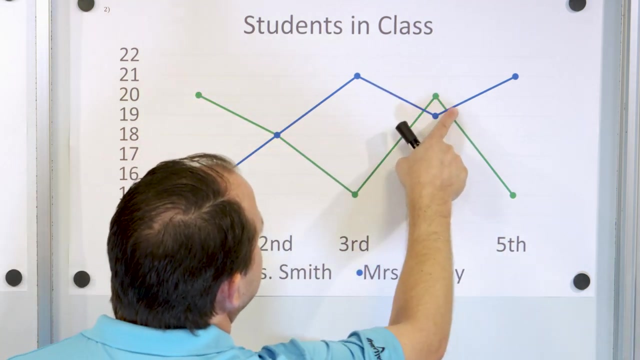 to that over here on week one, And so you can use it to identify trends. All right, let's take a look at graph number two. We have the number of students in class over different periods of the day for two different teachers. So the green line like this: it goes down and up and then down, that's. 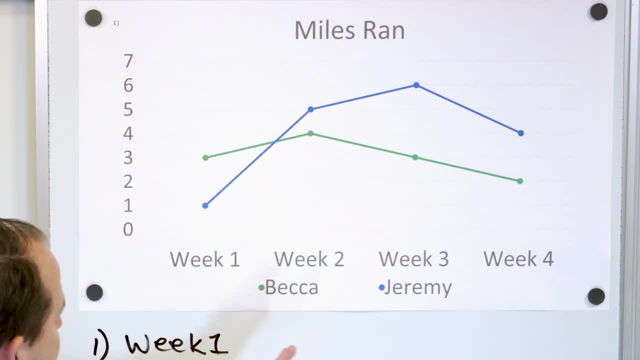 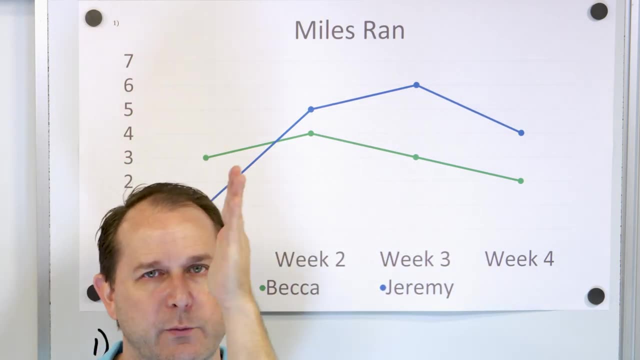 is happening. Week two: you go up, read these numbers, That is what is happening. Week three: you go up, This is what is happening, and so on. And so if you isolate it to week one and two and three and just look at what's happening on those weeks, then it makes more sense. And 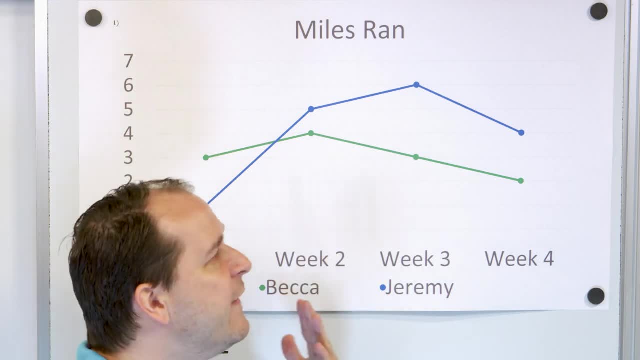 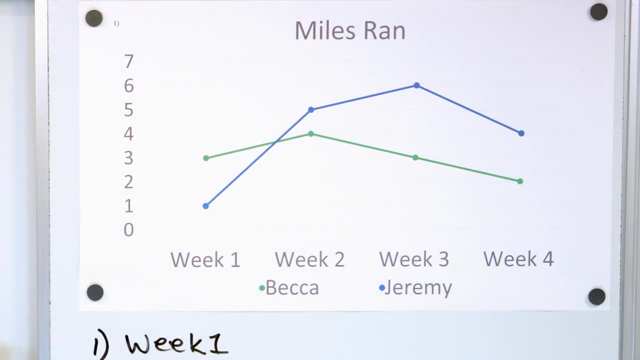 you can use the connection of the lines to get an idea of the trend. You can see that in general, Jeremy runs more often or more miles than Becca- But of course there's an exception to that over here on week one- And so you can use it to identify trends. All right, let's take a look. 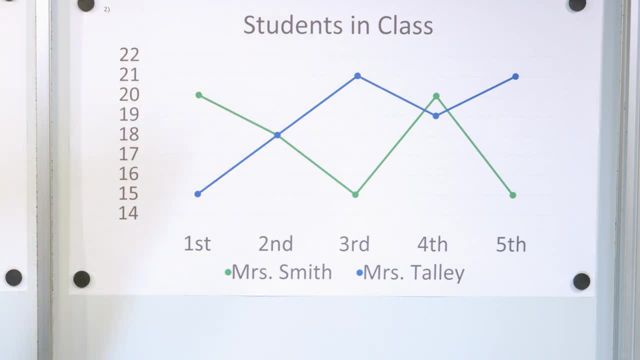 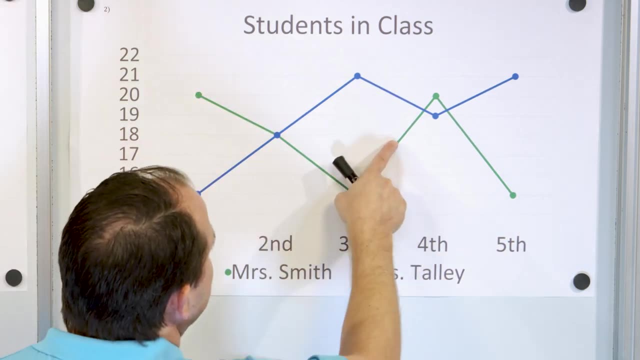 at graph number two, We have the number of students in class over different periods of the day for two different teachers. So the green line, like this, it goes down and up and down. That's Miss Smith And this is the number of students in class over different periods of the day for two different. 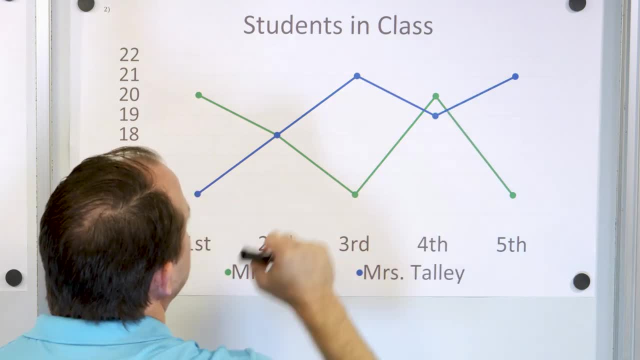 So the green line, like this, it goes down and up and down, That's Miss Smith And this is the number. Then the blue line is Miss Talley. It goes up and then down and then up, like this. And the way you read this thing is you say: well, each of these teachers have first period, second period, third, 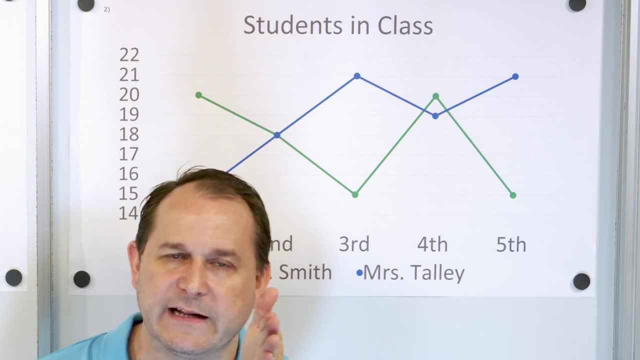 period, fourth period and fifth period: Same thing. First, isolate your gaze to first period, First period. what is happening? Miss Talley, has you read it over? because Miss Talley is in blue is 15 students In first period. Miss Smith in green is a lot more students at 20.. Now 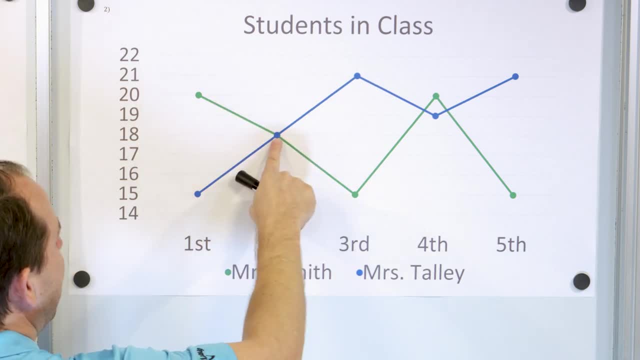 in second period. it looks like the graphs cross. Both of the different teachers actually have 18 students for second period, But by third period everything reverses and the blue graph is on top. Miss Talley has 21 students and Miss Smith. 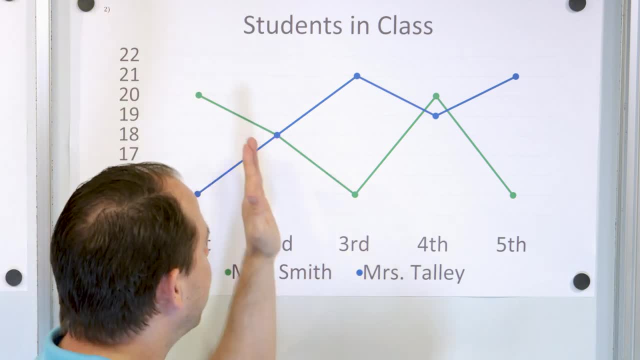 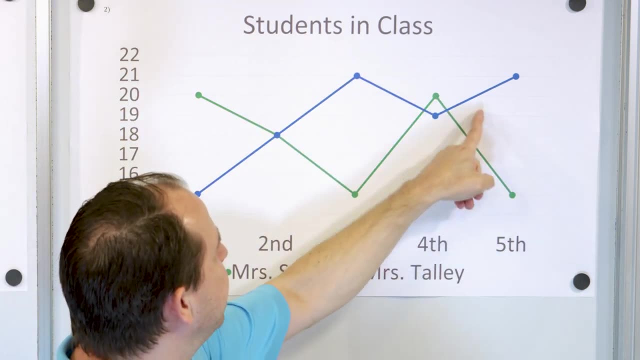 has gone down to 15 students and so on and so forth. So you go in time, or in this case in period one, period two, period three, and just read up and see what's happening. Read up and see what is happening, You can see that by fifth period Miss Smith again only has 15 students. 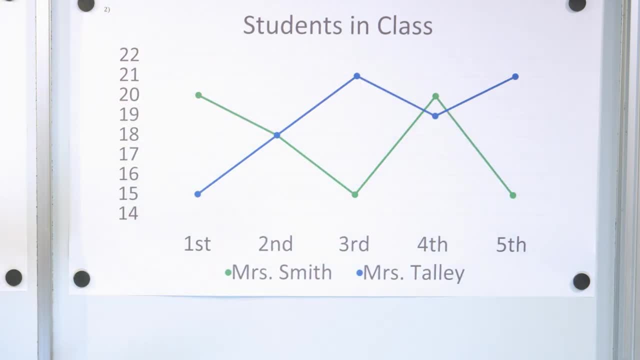 but Miss Talley has 15 students, So you go in time or, in this case, in period one, period two, 21.. So let's read question number one and try to answer the questions. During what period does Miss Smith have the fewest students? So when you're looking at Miss Smith, you only look at 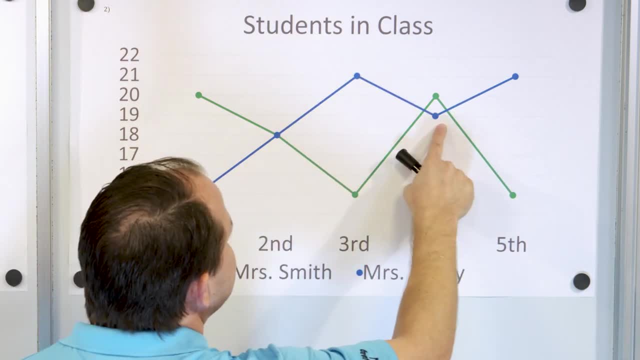 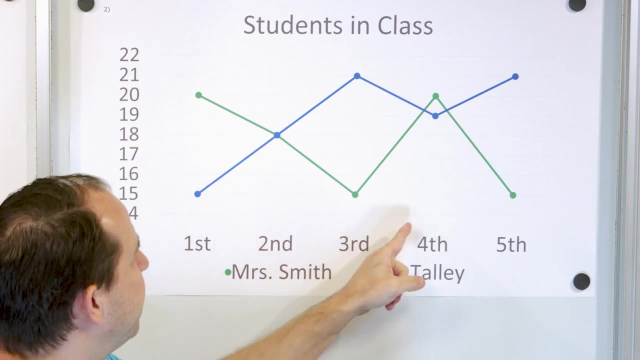 Smith, And then the blue line is: Ms Talley goes up and then down and then up, like this. And the way you read this thing is you say: well, each of these teachers have first period, second period, third period, fourth period and fifth period. Same thing. First, isolate your gaze to first. 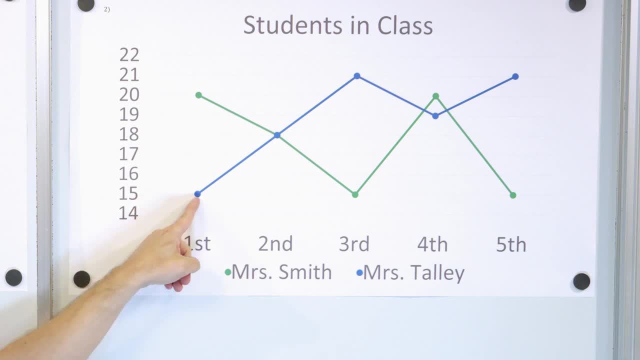 period, First period. what is happening? Ms Talley- has you read it over? because Ms Talley is in blue- is 15 students In first period. Ms Smith in green is a lot more students at 20.. 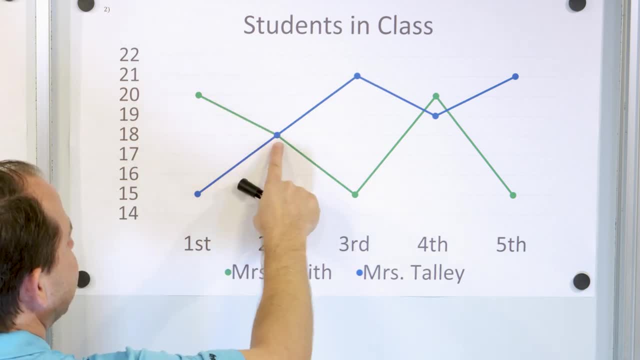 Now in second period it looks like the graphs. they both- both of the different teachers- actually have 18 students for second period, But by third period everything reverses and the blue graph is on top: Ms Talley has 21 students. 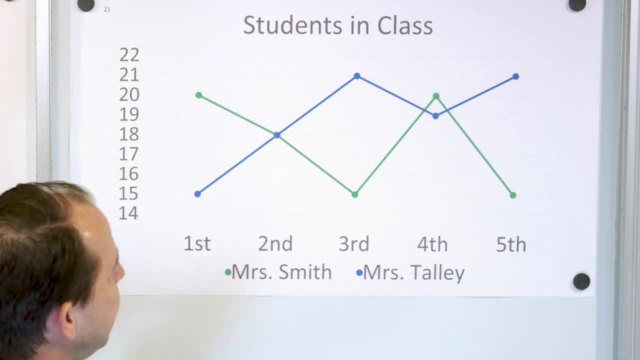 and Ms Smith has gone down to 15 students and then and so on and so forth. So you go in time, or in this case, in period one, period two, period three, and just read up and see what's happening. 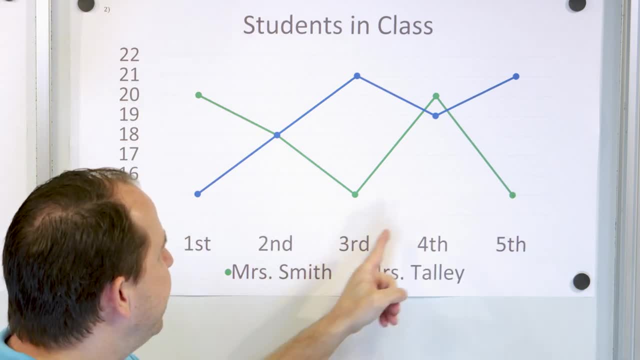 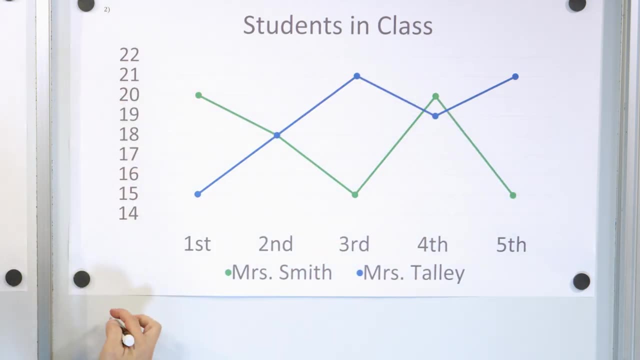 Read up and see what is happening. You can see that by fifth period Ms Smith again only has 15 students at 21.. So let's read question number one and try to answer the questions. During what period does Ms Smith have the fewest students? So when you're looking at Ms Smith, you only look. 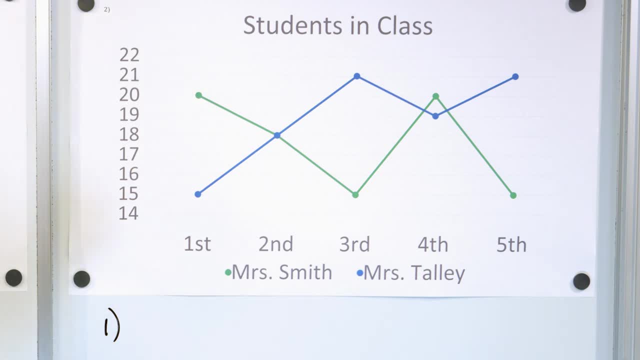 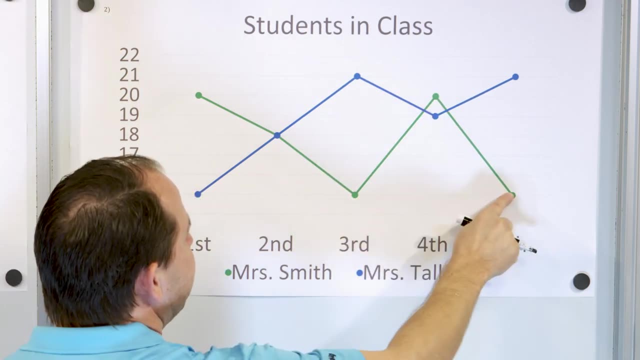 at the green line. You ignore everything else. What period does she have the fewest students? Well, that's not the fewest. That's not the fewest. That looks to be the fewest, That's not, but these two were tied. You see, these are the exact same number: 15 students. So third period. 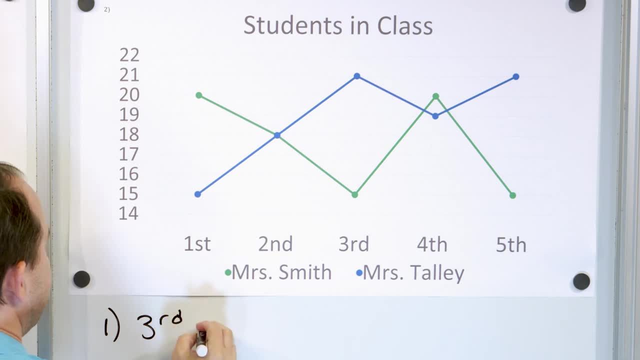 and fifth period. Third and fifth Period. In other words, both of those periods are tied, but the fewest number of students from Ms Smith and the number of students in those periods is the lowest she has during the day, which is 15 students, All right. Problem number two: who has the most students over the five? 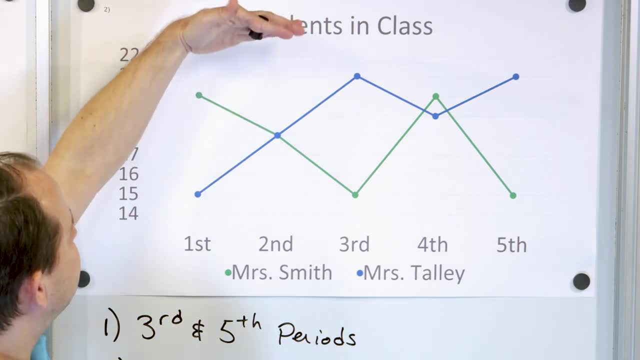 periods. Who has the most students? Well, you basically look at the top of the graph. You have the green. the highest place the green gets is 20 students. The highest place Ms Smith and green gets here is again 20 students. 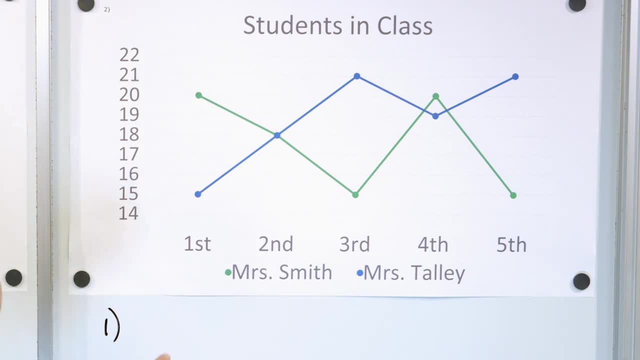 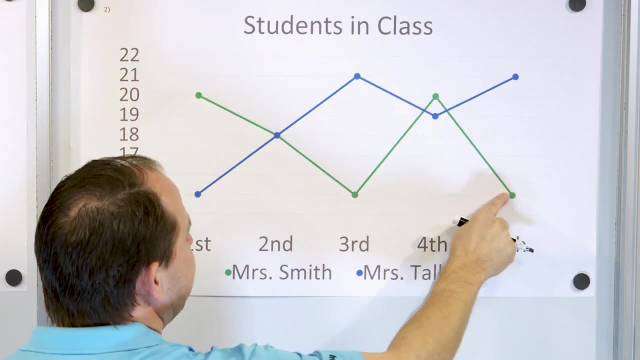 the green line. You ignore everything else. What period does she have the fewest students? Well, that's not the fewest. That's not the fewest. That looks to be the fewest, That's not, But these two are tied. You see, these are the exact same number: 15 students. So third period and 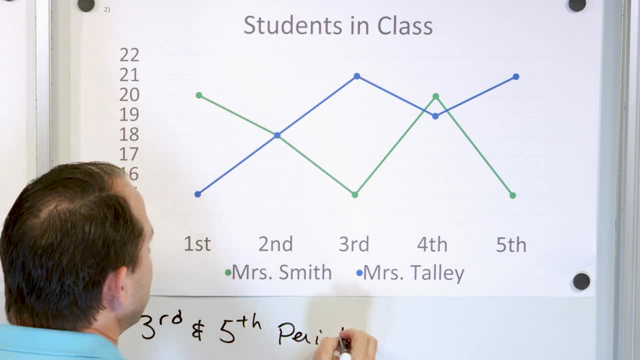 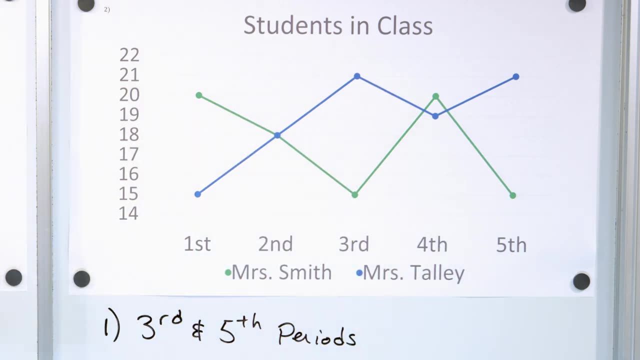 fourth period. In other words, both of those periods are tied, but the fewest number of students from Miss Smith and the number of students in those periods is the lowest she has during the day, which is 15 students, All right. problem number two: Who has the most? 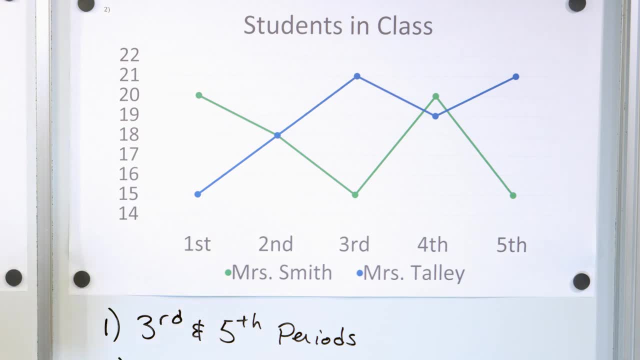 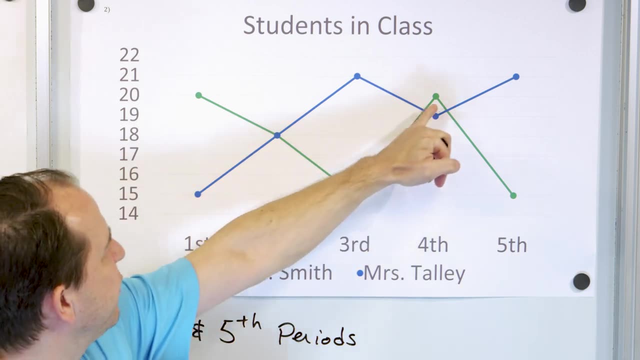 students over the five periods. Who has the most students? Well, you basically look at the top of the graph. You have the green. The highest place the green gets is 20 students. The highest place Miss Smith and green gets here is again 20 students. But Miss Smith has the most students. 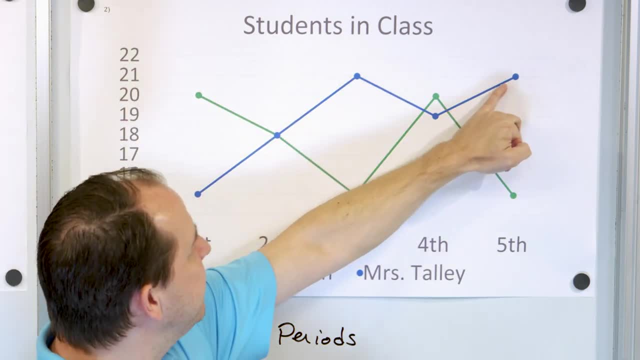 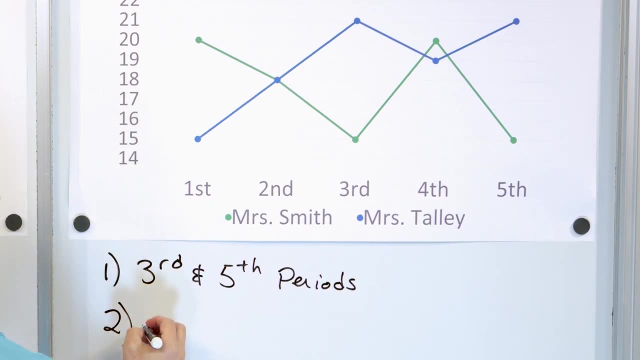 Miss Talley gets to a maximum of 21 students, And again in fifth period she gets down again to a maximum of 21 students. So who has the most students throughout the day? It's going to be Miss Talley, And again she has two different periods that have the same number of students, which is 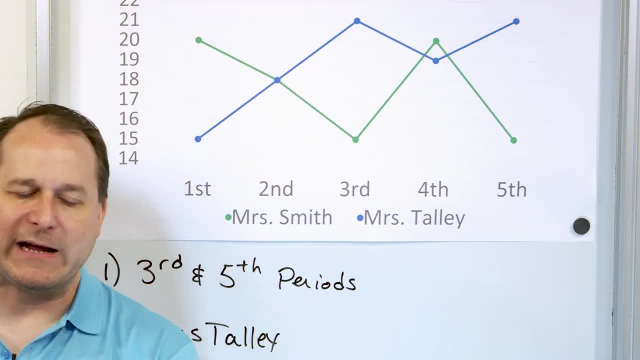 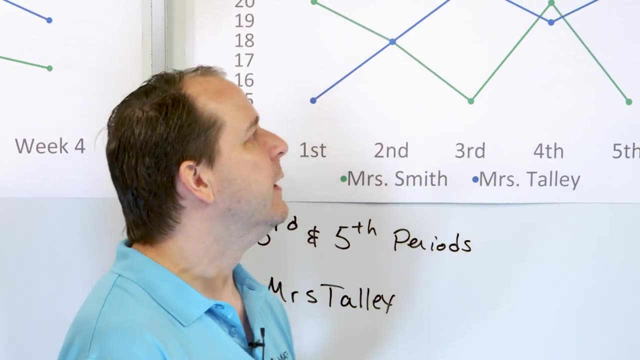 her maximum at 21.. So again, we're just getting practice learning how to read line graphs. I'd like you to go through them, Really study them. Don't just answer the questions I put, but just make sure you understand what the graph is telling you. I mean what this graph is telling. 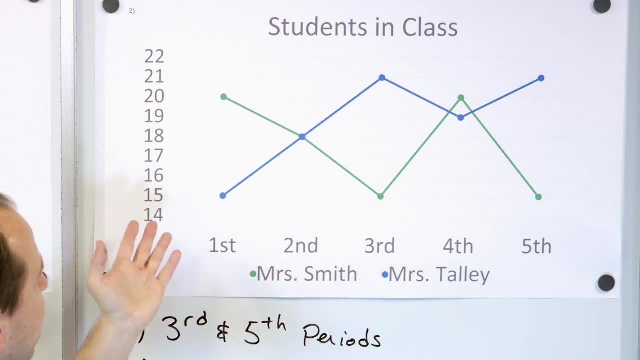 me in general is that Miss Talley has more kids in general, because here she has a lot of students and then a little bit less and then a lot more. But then of course in the beginning, in the early morning hours of the day, in first and second period she has significantly fewer students. 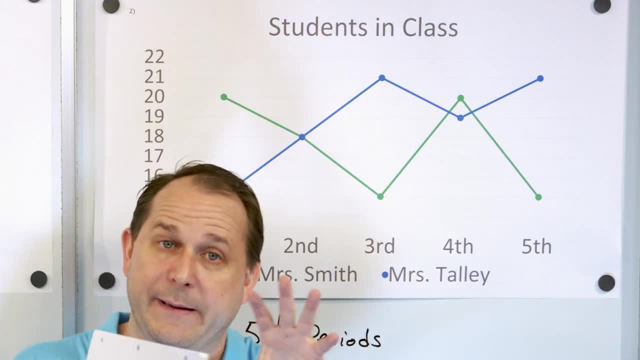 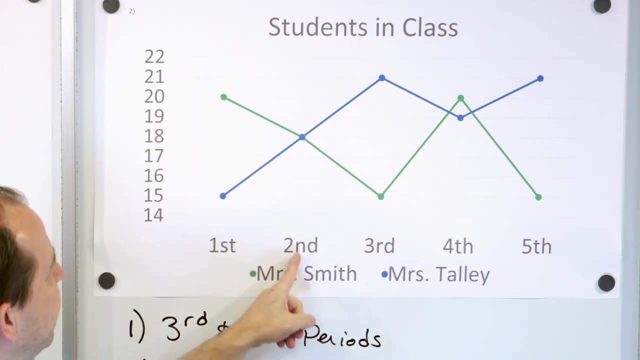 So you can read it different ways. You could look at how they're compared together, or you can just look and see how their day is looking as far as number of students throughout the day. The green line- here Miss Smith- is all over the place throughout the day, whereas the blue class. 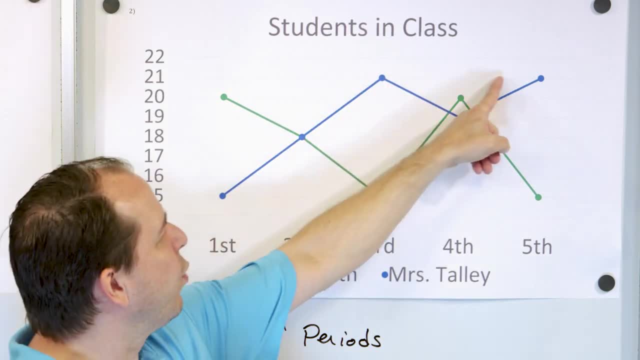 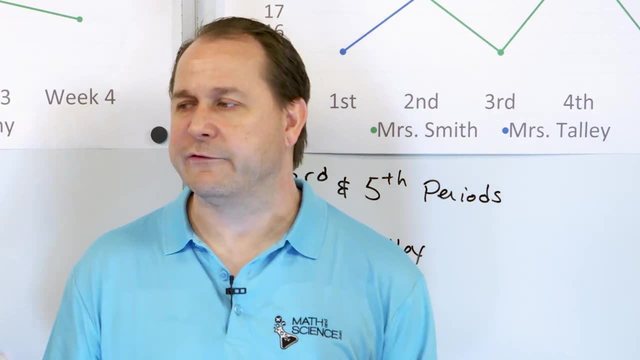 the blue line here. Miss Talley looks like she has fewer students in the morning but then more students in the afternoon, So you can use it to find trends. I'd like you to go through this yourself. Make sure you can understand and answer these questions. Follow me on to part two. We'll wrap up the concept of line graphs.